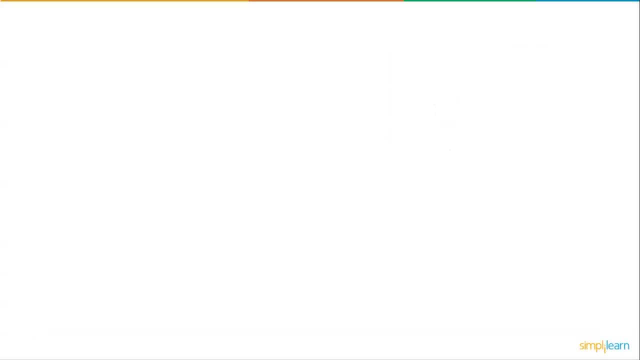 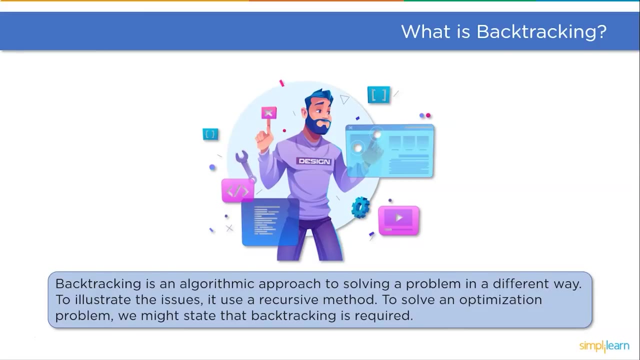 from Simply Learns YouTube channel. So, without any further ado, let's get started with an introduction to backtracking. Backtracking is an algorithmic method of alternately solving a problem. To explain the issues, it employs a recursive approach. Backtracking is required to find: 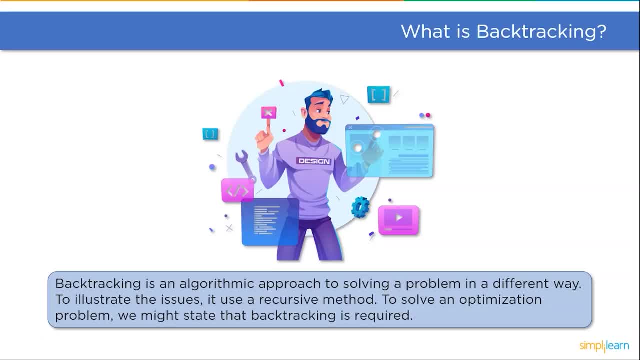 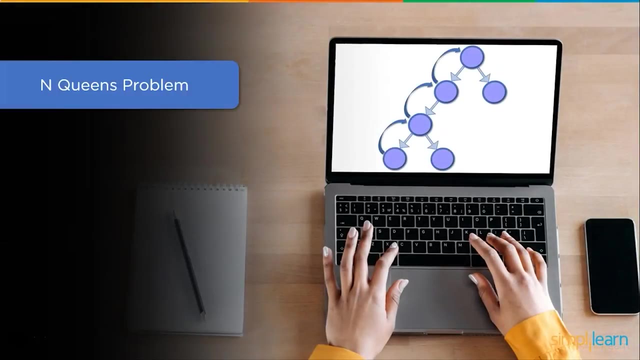 every possible combination to solve an optimization problem. Backtracking is used in solving various problems like nQueens, Night store, the rat in the maze problems, and so on. Now, to get better understanding of backtracking, let's have a brief look at nQueens problem. 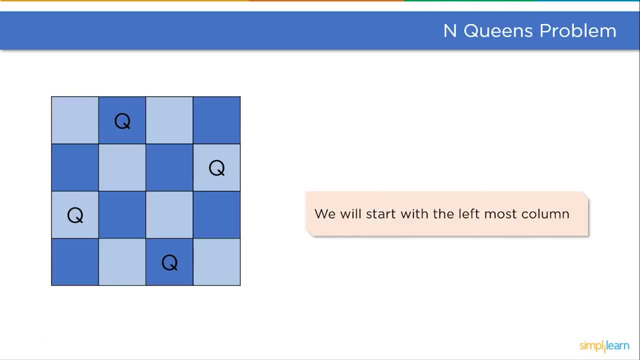 Let's say we have 4x4 matrix, We have to place 4 queens in that Every row and column has exactly one queen and none of them falls under the same diagonal. We will start with the left most column, Then we will check our base condition that if we have placed all the queens or not, Now we 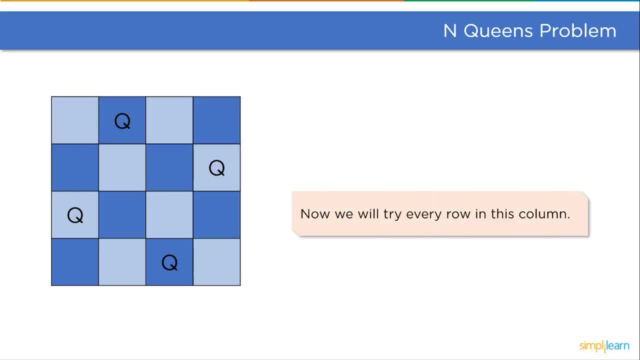 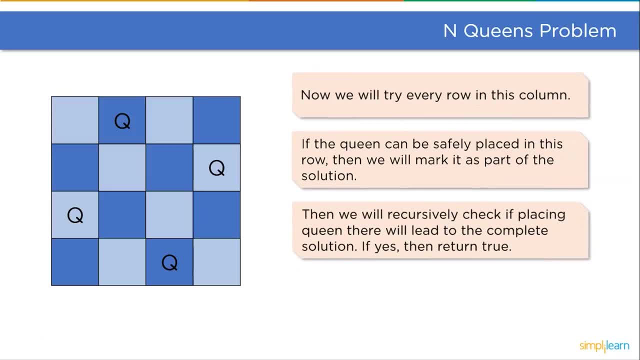 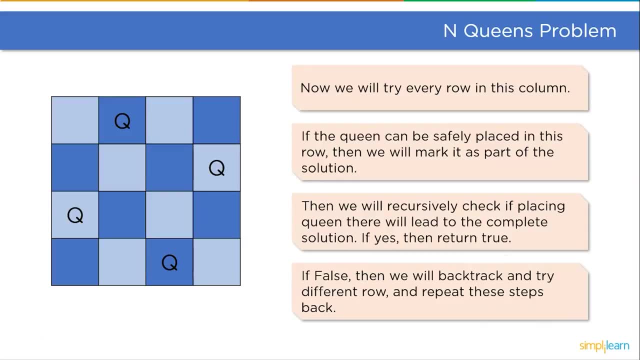 is a very simple method. We will specifically check if placing queen here will lead us to the solution or not. If yes, then we will return true. Otherwise, if false, then we will backtrack and try other rows and repeat these steps If all rows have. 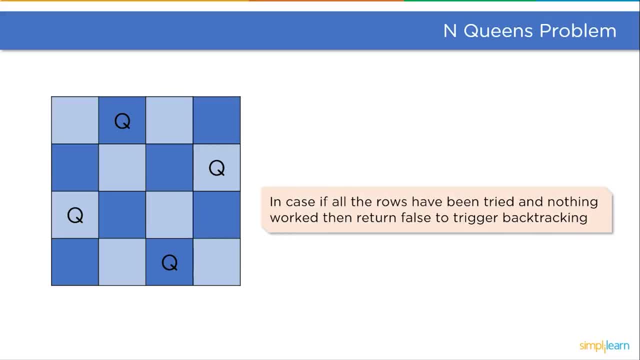 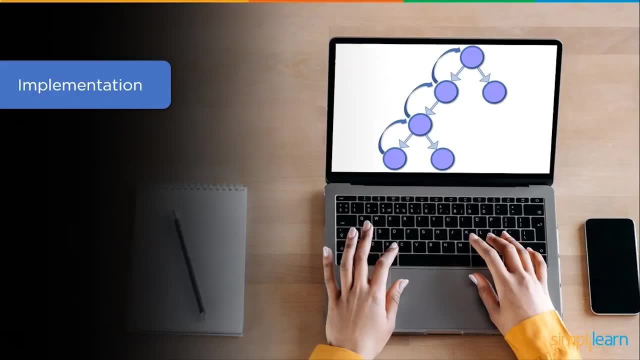 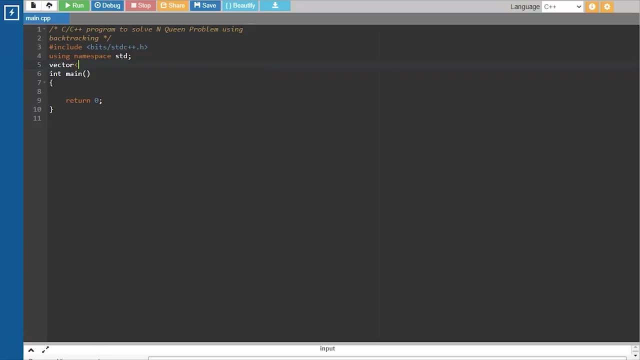 tried and nothing worked, then I will return false to trigger backtracking. Now let's implement this nQueens problem in the coderator. We will define a vector inside a vector. it will be a int vector. result: now we will write a utility function to check if the queen can be placed on board. 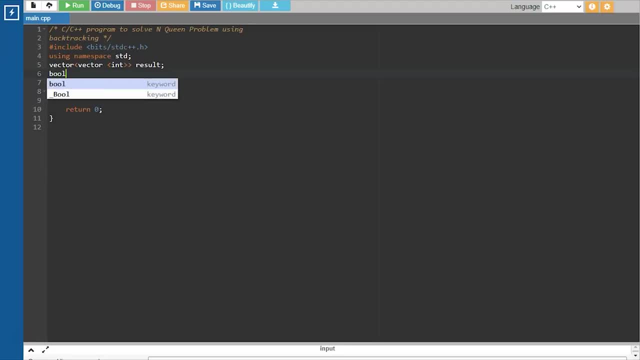 so it will be a boolean function. bool is safe as argument. we will place a vector inside a vector: int bool, comma, int row, comma, int column. we will define int i, comma j. int n will be equal to board size. now we will check if this row on the left side 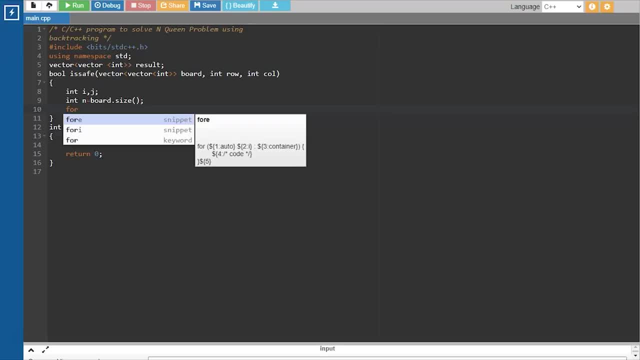 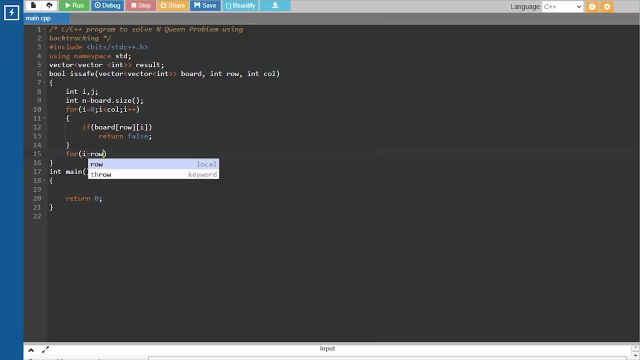 i, i, j, j, j greater than equals to 0. i j greater than equals to zero. i i greater than equals to 0. i, i, i, i, j, j, j minus minus f. board i comma. j then return. now we will check lower diagonal on left side. 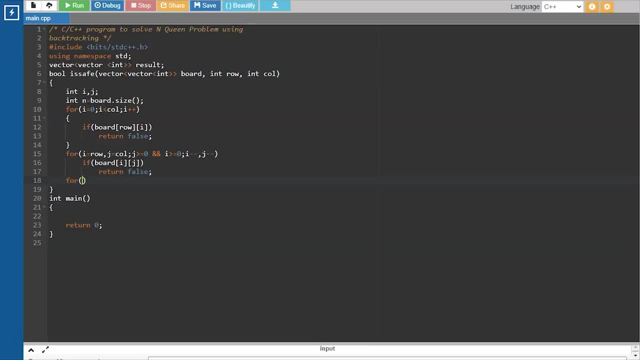 so for i equals to row, comma, j is equals to column, i less than n and j greater than equals to zero. i plus plus comma, j minus minus. now, if board at i and j will return, else we will return j and j will return j, j, j. 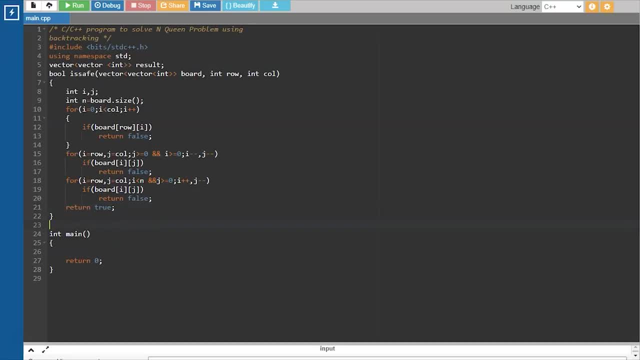 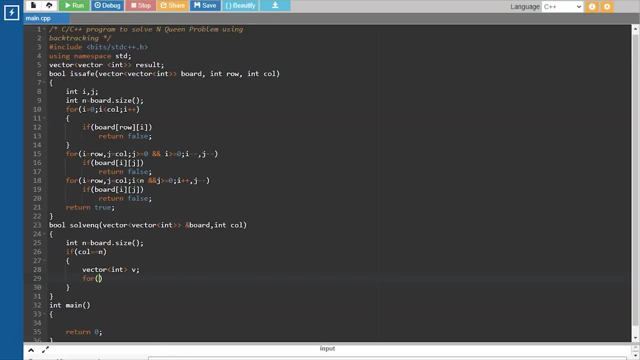 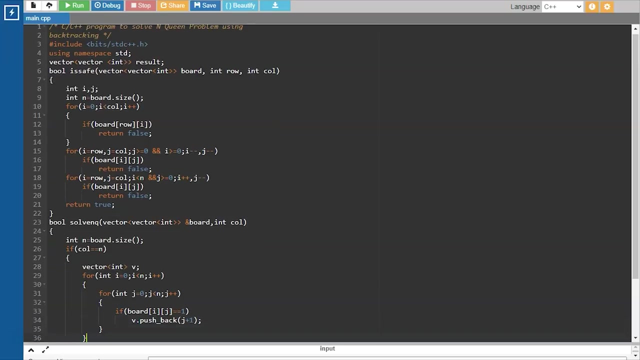 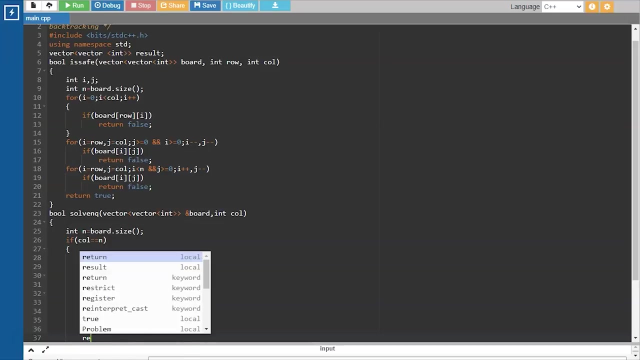 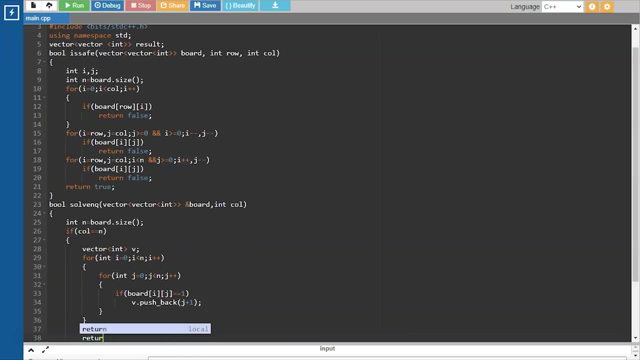 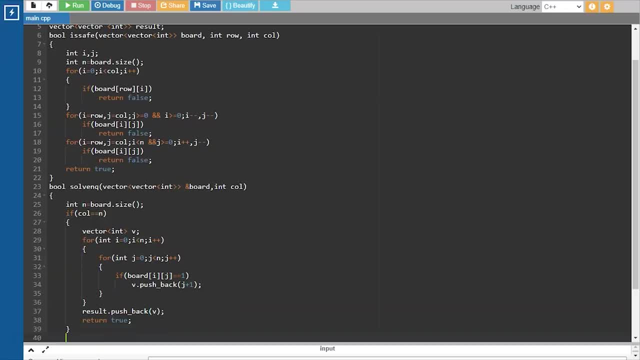 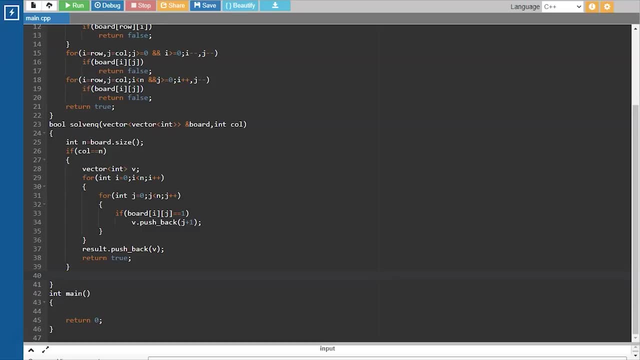 Now we will consider this column and try placing this queen in all rows one by one. So boolean does is equals to false. Now for loop print: i is equals to 0,. i less than n, i plus plus. Now we will check if queens can be placed on board i and column call. 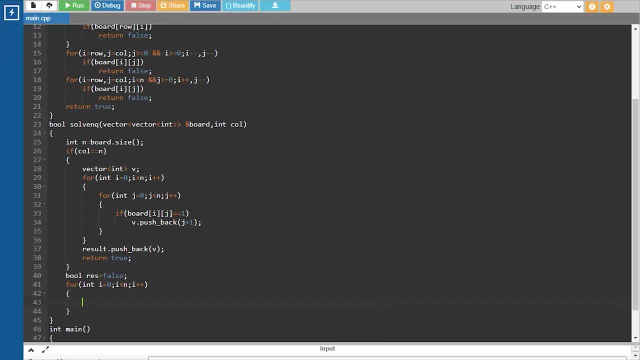 So if Is safe, board comma i comma call. If it's safe, then we will Place this queen at that position. so board i call is equals to 1. Now we will make result true if any placement is possible. 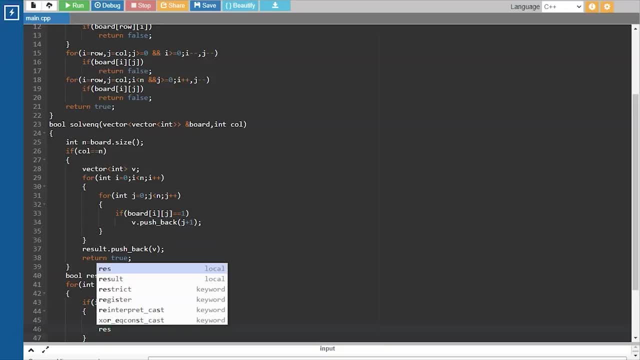 So res is equals to solve and queue. Now we will write call at board comma, call plus 1 or res, So res is equal to zero. Now we will make the queue. Now, if placing queen in board i call doesn't lead to a solution, then we will remove the. 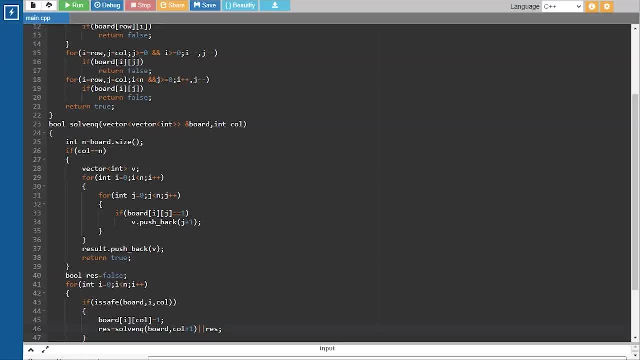 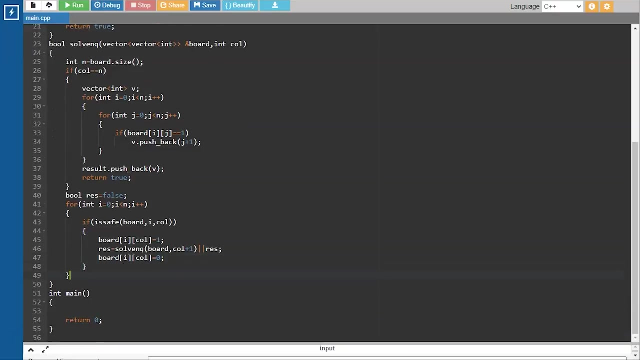 queen from the board i column and backtrack. Now, if queen cannot be placed in any row in this column, then we will return false. So return false Now. this function solves the error. Now, if queen cannot be placed in any row in this column, then we will return false. 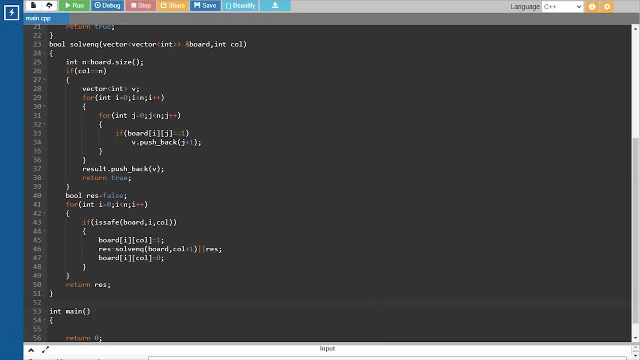 Hence we will solve the N행queen's problem using backtracking. It is basically using SOLVE NQ to solve problem. it returns false if queen cannot be placed otherwise, returns true and print placement of queen in the form of ones. Now there may be possibility that there are more than one solution. 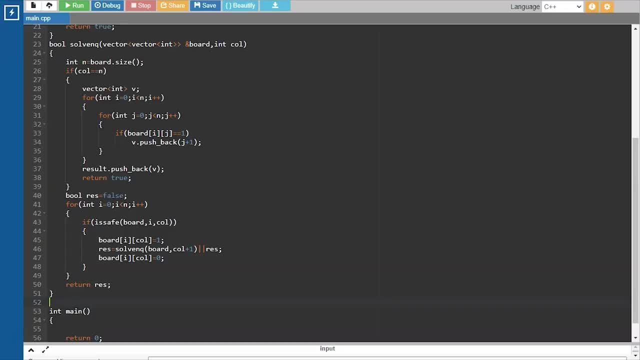 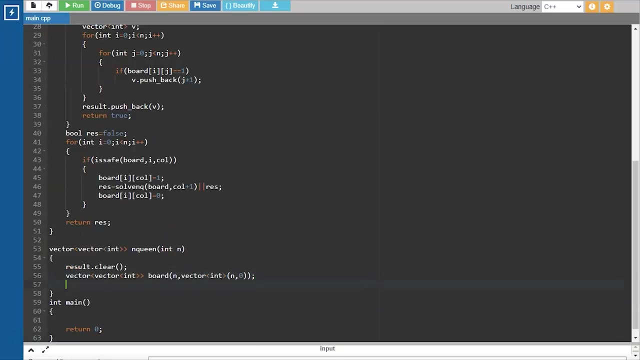 Then this function will print one of the feasible solution: Ida, vector and queen and n resultclear. now we will call vector inside a vector board, nvector, int and bracket. now if solve nq at board is false, then we will return empty set. 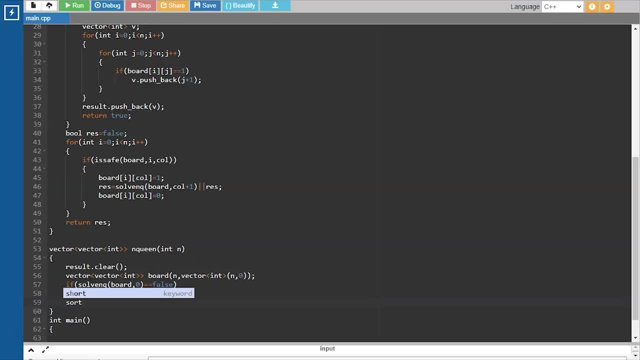 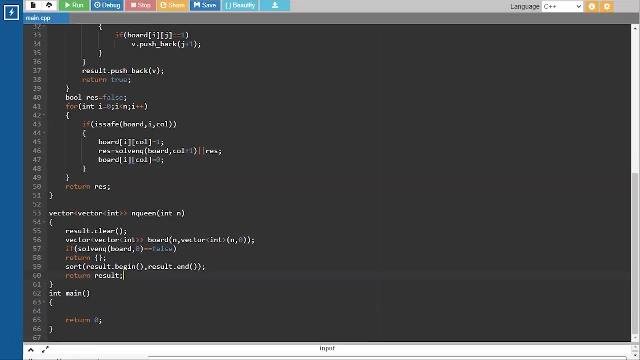 otherwise we will sort result: dot begin, comma, result dot end and we will return result. now we will write the main block, so int n is equals to 4, so for vector inside vector int v will be equals to n, queens at n. so we will write for loop. 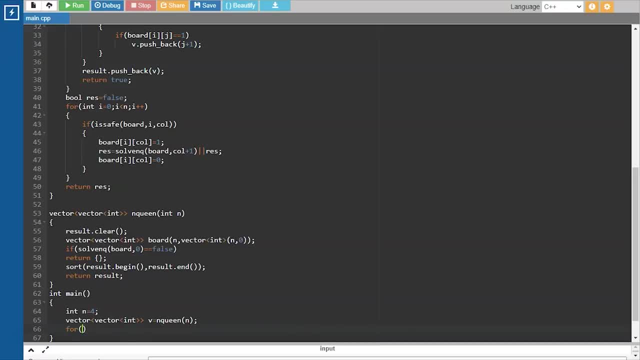 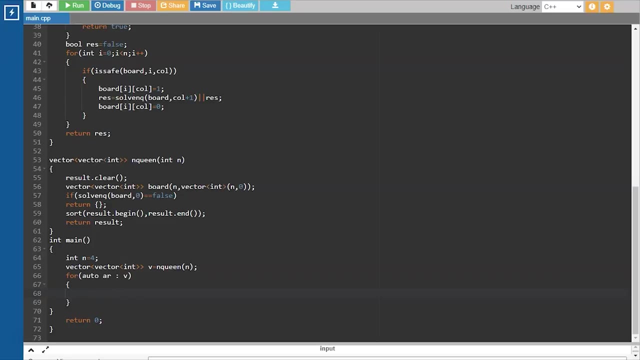 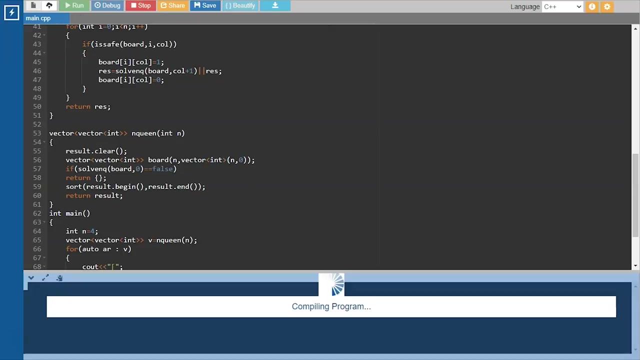 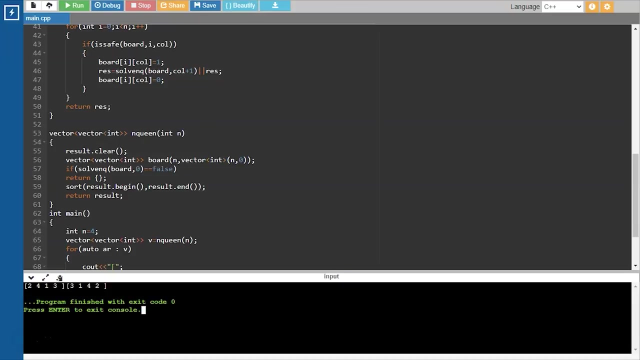 auto, auto, auto, ar, auto, ar v. we will call cout. we will call cout, then for loop: Auto, ATR, AR, see out ITR and see out, and then we will return zero. now let's run this code. as you can see, we are getting two answers. now this end queen can be solved with both of these answers.